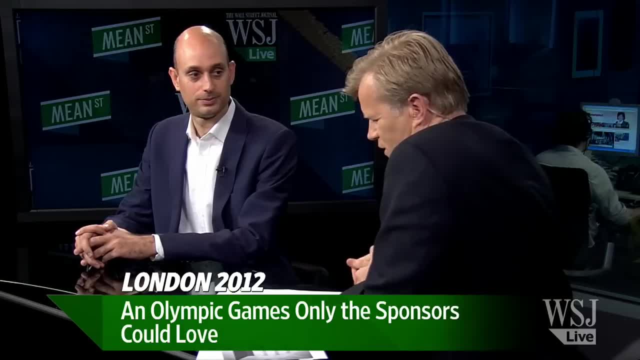 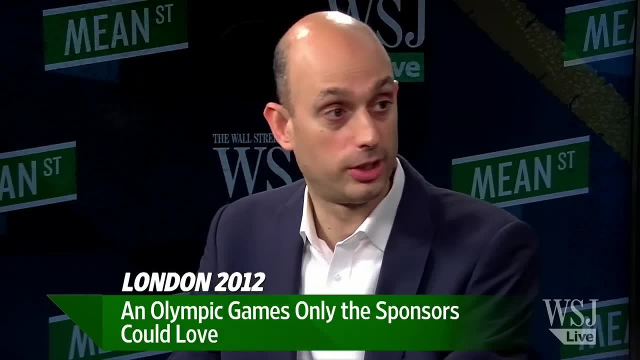 Sam Mahmoodi from Market Watch sports columnist at Market Watch, here to talk about this. What's going on? There was a minor controversy last week when Sebastian Coe, the great long-distance runner. he was also the chair of the organising committee. 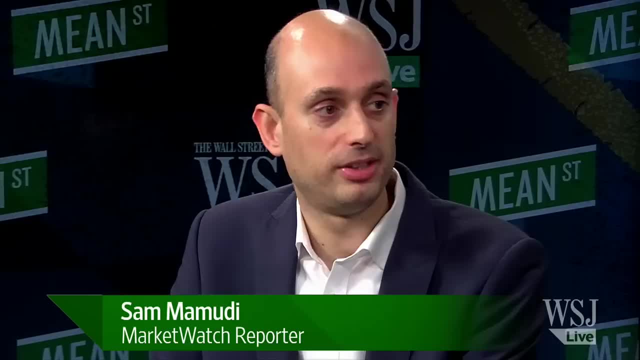 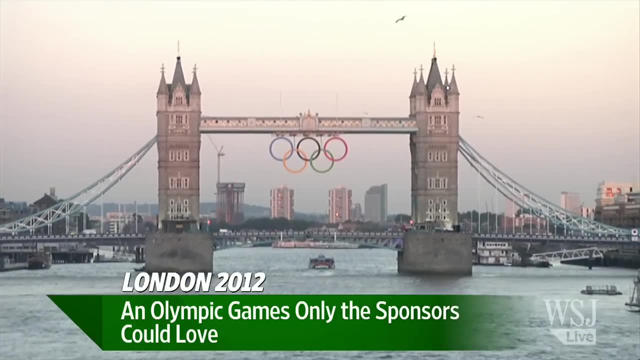 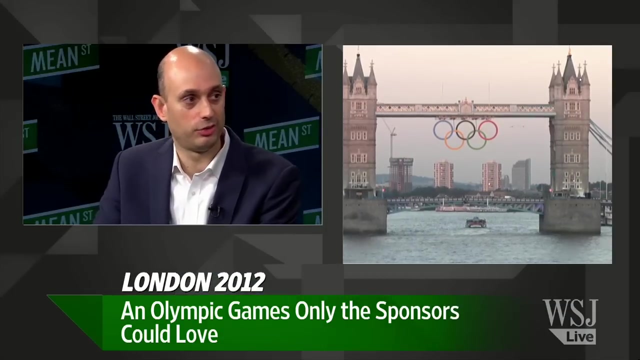 I think he perhaps misspoke, but he suggested if you were wearing a Pepsi t-shirt and you tried to go watch some of the events, you would get thrown out, Coca-Cola obviously being one of the Olympics' big sponsors. I think the issue is that in the UK and beyond, it kind of suggests that these games are very much about the sponsors as much as the athletes or us watching at home. 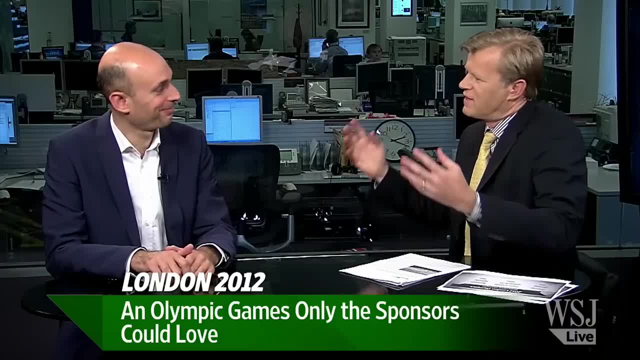 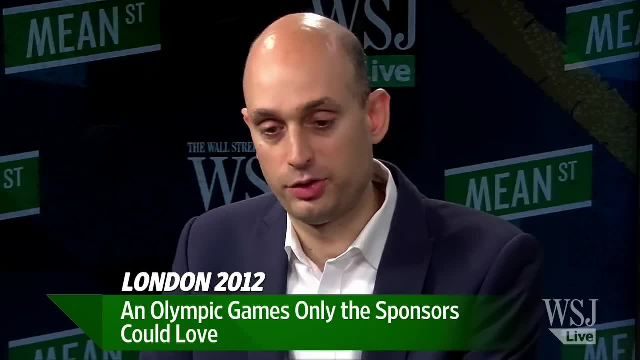 It's kind of unseemly to the average person. Obviously he has a much more romantic view of what sports are all about, right? Yeah, especially the Olympics, I think, because they were very much an amateur sport. they were all about competitive spirit. 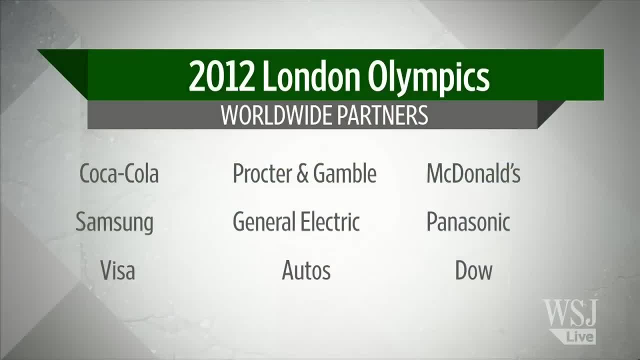 They have the Olympic Charter. Really, I defy you for the next two weeks, to watch anything to do with the Olympics. that is not going to be sodden in logos, Right? Well, that's the point. We're talking purely here about the sponsors. 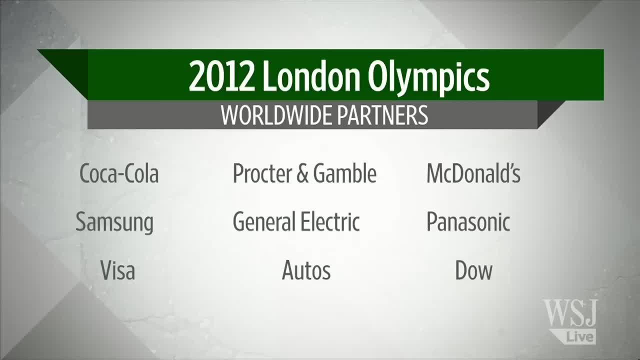 This is the London Organising Committee. They're sponsors. They have to obviously bankroll this enormous cost they have been putting on the game. They have to obviously bankroll this enormous cost they have been putting on the game. They have to obviously bankroll this enormous cost they have been putting on the game. 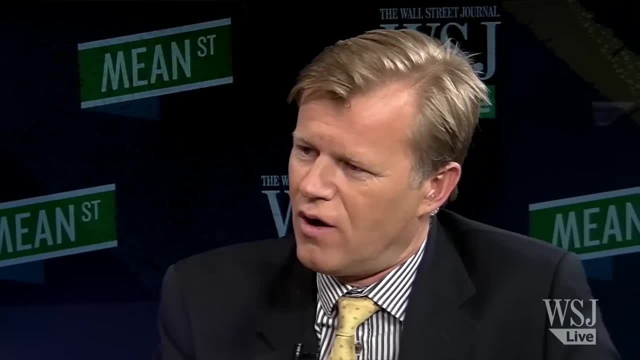 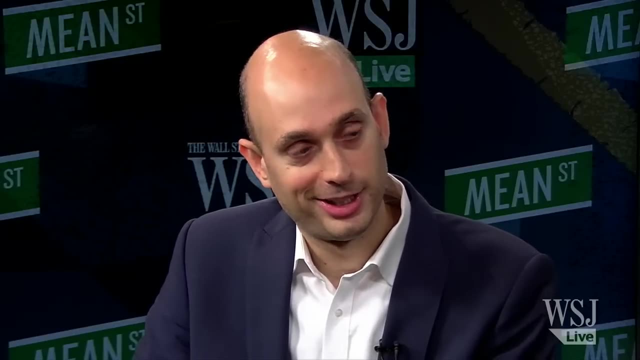 But players are allowed to carry the logos, are they not of their own individual sponsors, correct? You can, except for just before, during and just after the games. You can't be in any advertising or do any marketing if you're a Nike athlete. 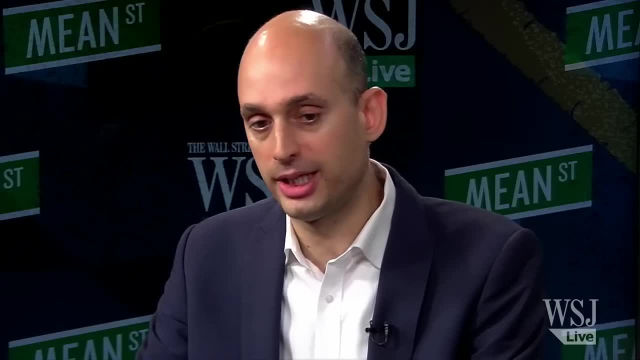 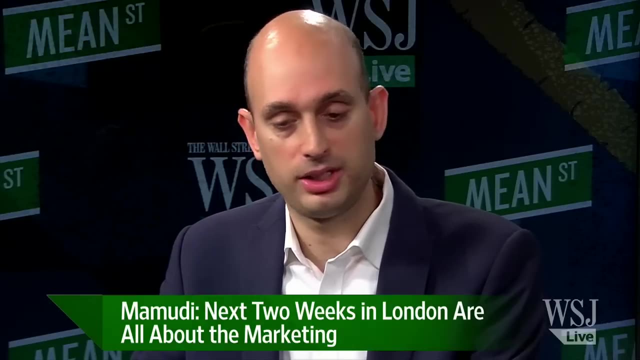 Adidas are the big sponsors for the Olympics, But you can wear Nike shoes. You can wear Nike shoes, but you're not going to see any Nike ads with any Olympic athletes going to be on. And that's kind of unprecedented When you think about it. if the Super Bowl is on and Peyton Manning is in it, 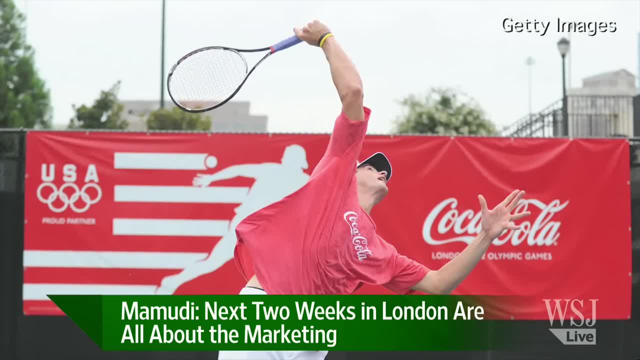 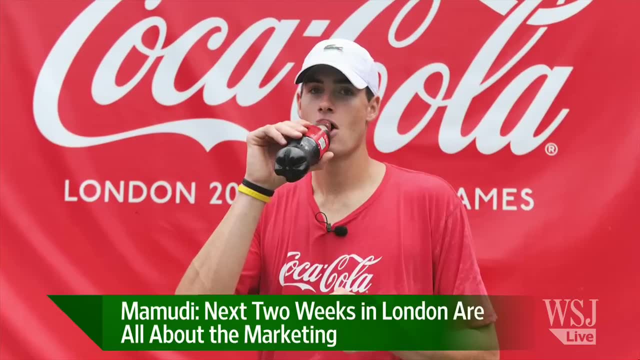 we're going to be flooded with Peyton Manning ads for every single product he can get his hands on and endorse. But that's the weird thing of harking back to the amateur ideal but at the same time serving the people, who pay about a billion dollars every four years. 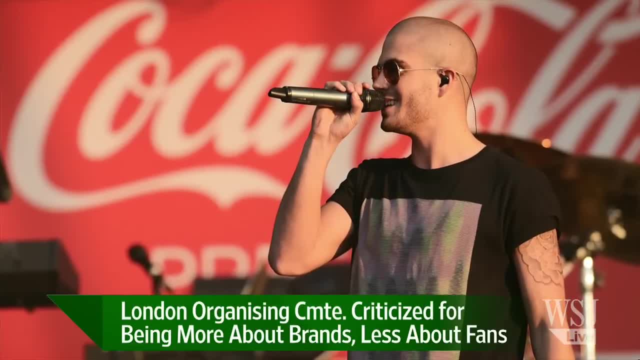 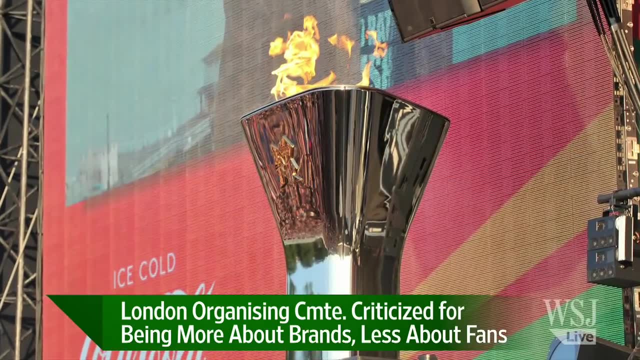 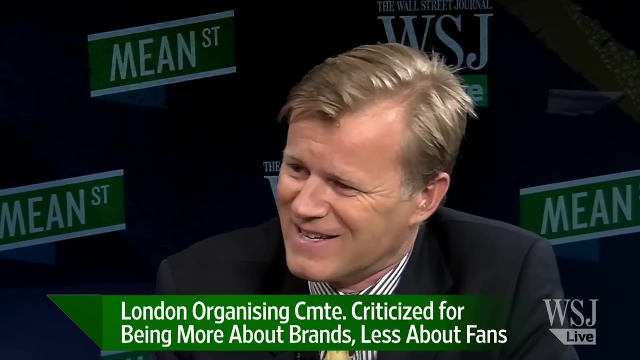 Right, right. So yes, it's kind of like trying to have your cake and eat it too. perhaps They are having their cake and eating it. They are indeed eating a lot of it, perhaps, But some other stories. I read something the other day about some butcher who had put the rings in the shape of sausages, or something like this.